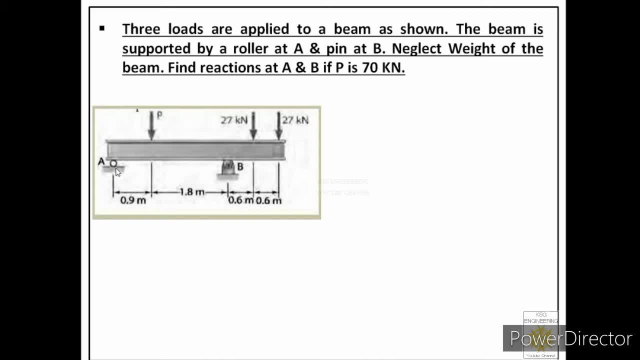 first locate the reactions or the constraints provided by these reactions. So we are asked to find the reactions of the beam moving at different points in the A and B axis. Here again we are given two measures by which the Canon sp can be Squeeze. 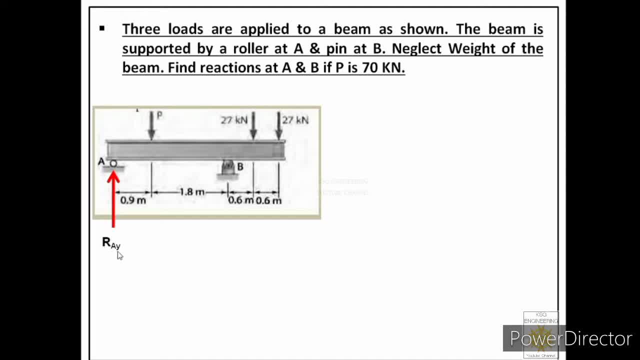 and we have labeled it as reaction at A in Y direction, then at B. we have to label two constraints, one normal to the surface, one along the surface. so we have labeled it as reaction at B in Y direction, reaction at B in X direction. now one thing to understand over here, that at the start we don't know the. 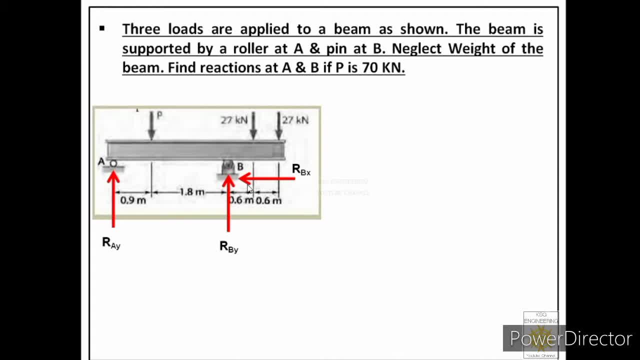 directions of these constraints or these reactions. we have just assumed that these two are acting in any other direction and this is acting towards left direction. fine, so when we get their answers, only then will come to know whether the directions assumed by us are correct or not. now we have made the free piped body, but one thing: 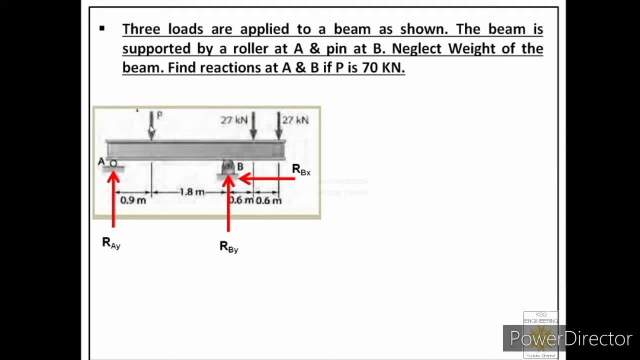 is missing. we have to label this P X as well. that is equal to 70 kN. Now free body is complete. So whenever you are solving such problems you should draw the free body first. That means whatever is given in the problem. draw that first, Then after that label the reactions at the supports and the external forces. 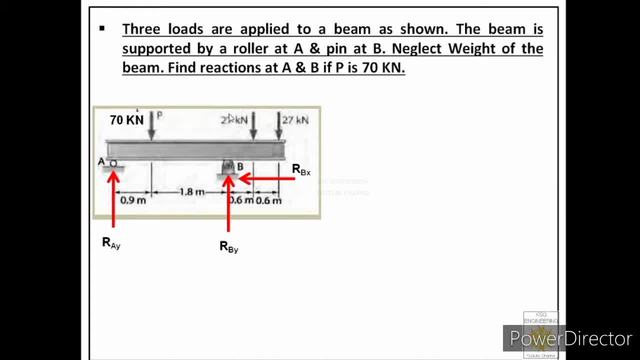 Now we know that this particular body is in equilibrium. That means we can apply three equations of equilibrium on this body. As body is not moving along x direction, then all the forces acting along x direction, their sum has to be zero. And we know body is also not moving in y direction. 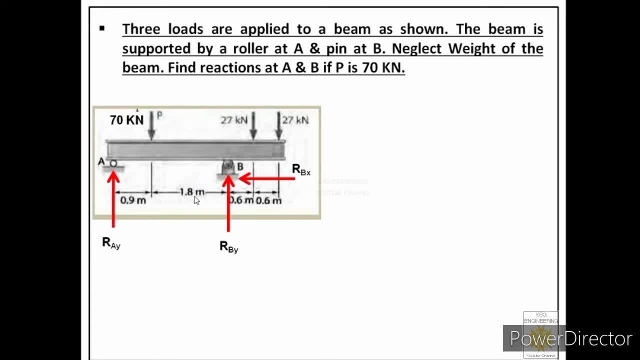 so all the forces acting along y direction, their sum has to be zero, must be equal to 0, as we know that this body is not rotating. that means the movements provided by all the forces about any particular point must be equal to 0. so let us apply the first equation, that is, summation: FX is equal. 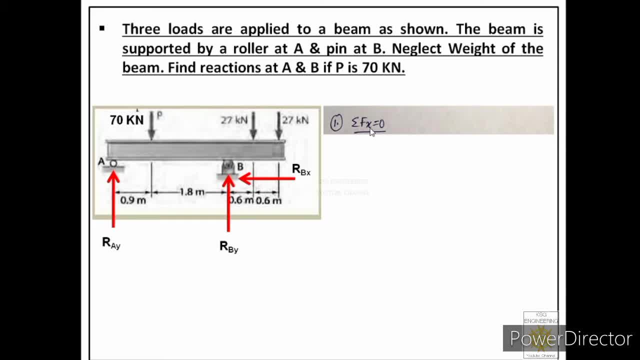 to 0. so let us see how many forces are acting in X direction. there is only one force acting in x direction, that is RBX. so from this we will get an equation RBX equal to 0. so we got our first answer, that RBX is 0. now let us apply the 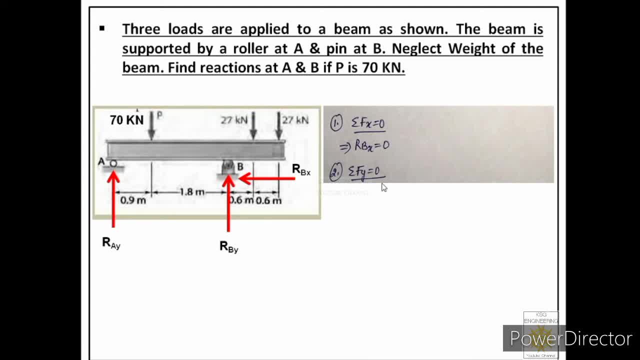 second equation, that sum of all the forces acting along Y direction is 0. so how many forces are acting in Y direction? 1, 2, 3, 4, 5. now the forces which are acting in downward direction. we will consider those forces negative, and the forces acting in upward direction will. 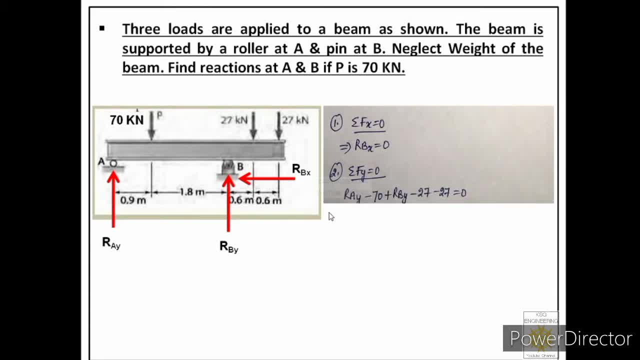 be considered as positive. so it means equation will become RAY minus 70 plus RBY minus 27 minus 27 equal to 0. so in this equation we have two unknowns. so we cannot solve this equation. so we will call that equation as equation number 1. 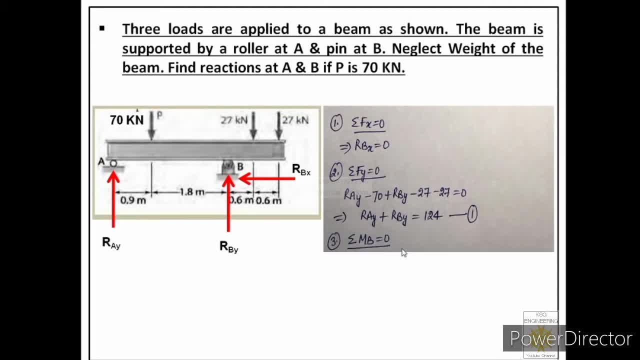 now we will apply the third equation, that is, movement of all the forces about any particular point must be equal to 0. in the previous numerical we have learned that we should consider that point as a movement center, at which maximum forces are acting, so that our equation should become simple. so let us take B as the movement center. so we are. 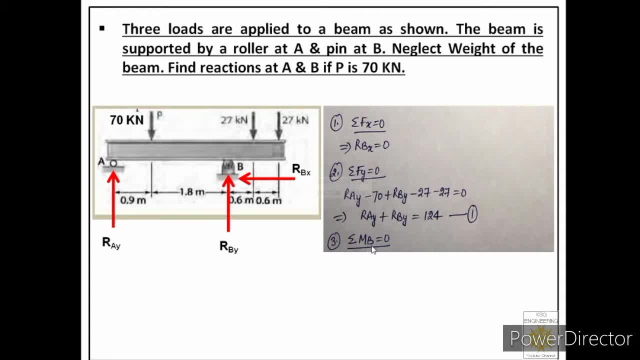 writing moments because of all the forces about point B must be equal to 0.. So let us see the moments generated by all these four forces about point B, because moment because of these two forces about point B will be 0, because their perpendicular distance from moment center is 0. So we will. 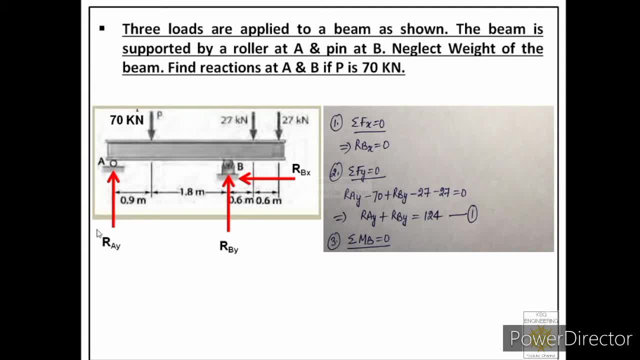 ignore these two. Let us first start with this force, Ray. Now, in order to find the moment of Ray about B, we have to first see its moment arm. So, for moment arm, what we will do, We will sketch its line of action. So this is the line of action, and from moment, 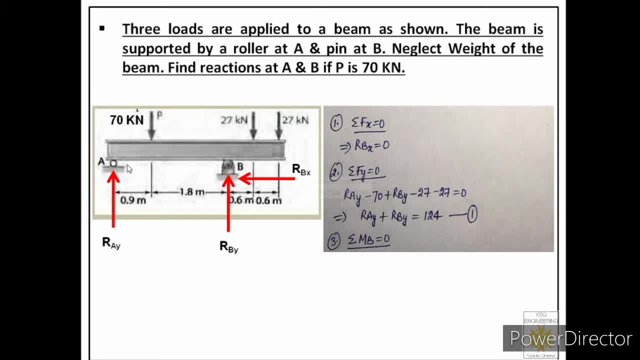 center. we will drop a perpendicular onto that line of action. So this moment arm is labeled over here as 1.8 plus 0.9.. So it is 2.7 meters. Next we will see the nature of the moment arm. So we will draw a line of action. So we will draw a line of action. 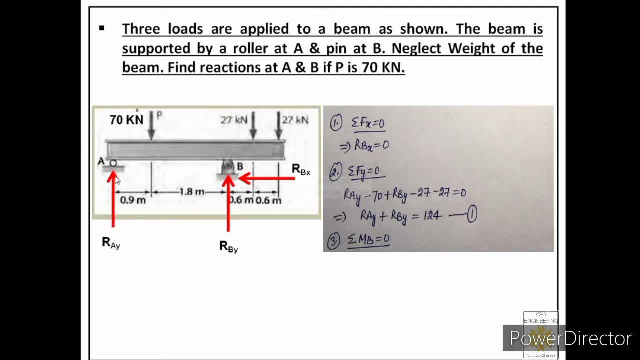 of the moment generated by this force. So this vector will try to move towards the moment center. So in that process it will generate clockwise moment. and we know clockwise moments are negative, So its moment will be minus Ray into 2.7.. Now let us talk about 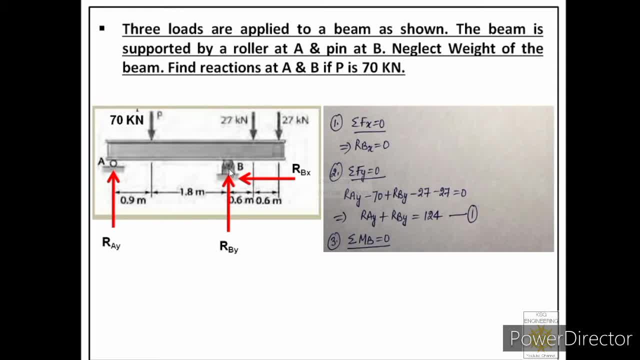 the moment because of this 70 kilo Newton force about point B. So first of all we will find its moment arm. So for that, first of all sketch its line of action. So this is the line of action of 70 kilo Newton force. Now, from moment center, drop a perpendicular. 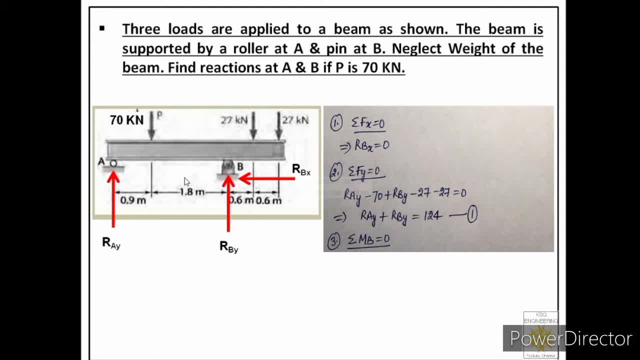 onto that line of action. So this moment arm is labeled over here as 1.8.. Next we will see its nature. So it will generate anti-clockwise moment. So this moment arm indicates that anti-clockwise moments are positive. So moment because of this force. 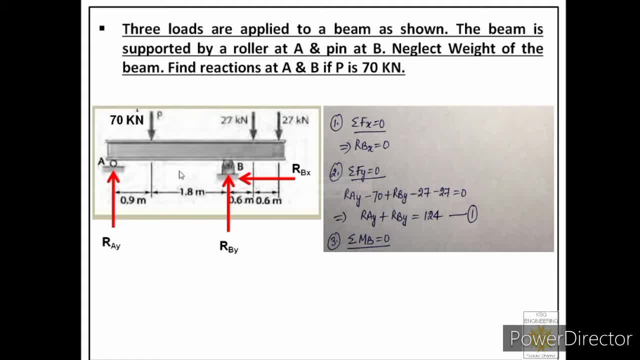 will be positive 70 into 1.8.. Next we will talk about moment because of 27 kilo Newton force, about point B. So this is the line of action of that force And when we will sketch perpendicular distance from moment center on 27 kilo Newton force, we will see. 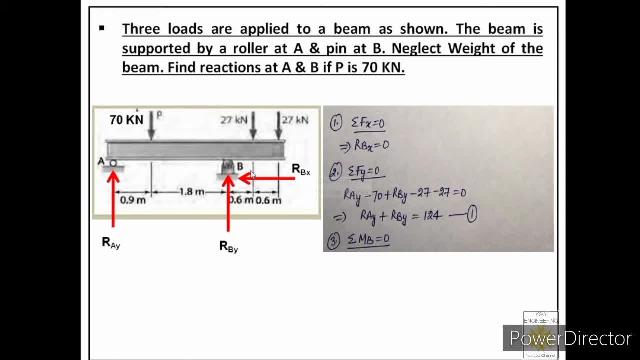 that moment arm is on to line of action, So that will be the moment arm. That moment arm is mentioned here as 0.6 meters. Then we will see the nature of the moment generated by this force. It will generate clockwise moment, and clockwise moments are negative. 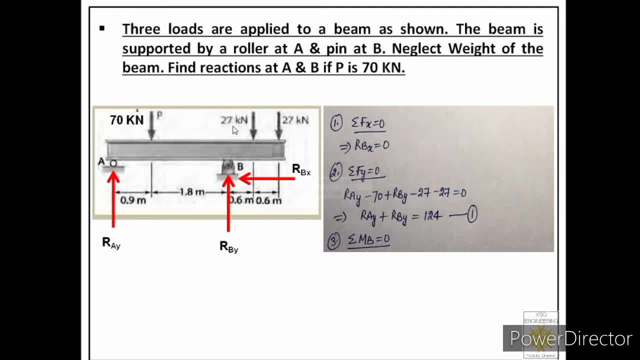 So moment, because of this force will be minus 27 into 0.6.. Now let us talk about the last force And this is the line of action of that force. From moment center, drop a perpendicular on to that line of action. So this moment arm is mentioned here: 0.6 plus 0.6, that is 1.2. 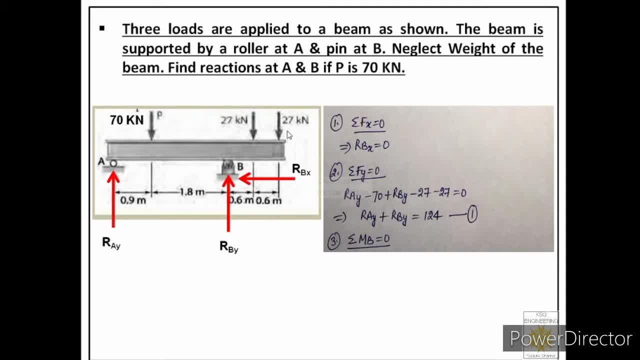 meters. And let us see its nature. It will also generate clockwise moment. So that is negative. So its moment will be minus 27 into 1.2 meters. So let us see this in calculations Over here you can see minus r ay into 2.7 plus 70, into 1.8 minus 27, into 0.6 minus 27. 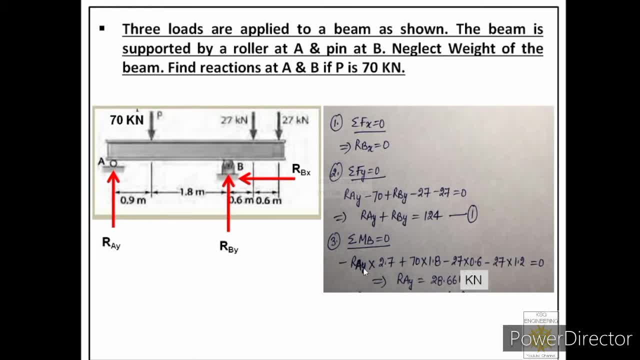 into 1.2 is equal to 0.. So in this equation we have only one unknown. So we can solve that unknown. Now you can see we got positive answer for that unknown. That means whatever direction we considered at the start of the numerical, that direction is correct Now. 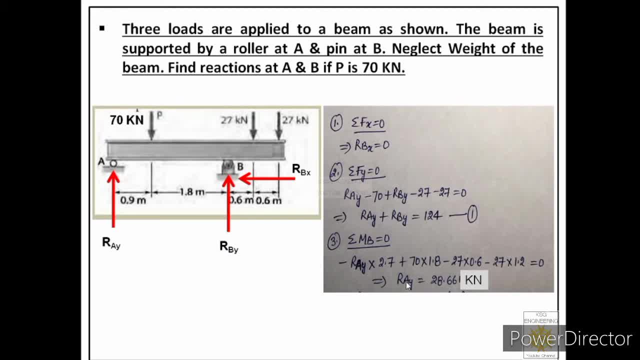 in order to find the second reaction, we will put this value in equation 1 to get the answer, And you will find that this particular reaction is also positive: Positive 95.33 kilonewton. That means the direction which we considered at the start of the numerical is correct. 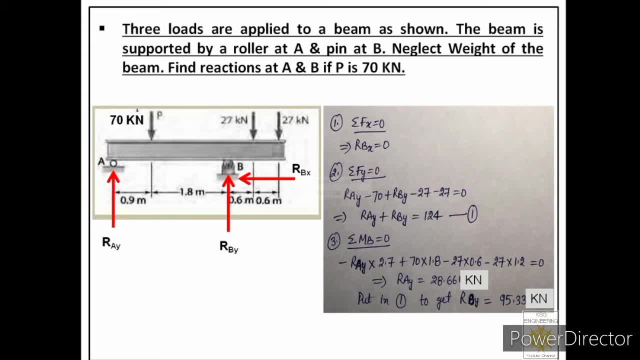 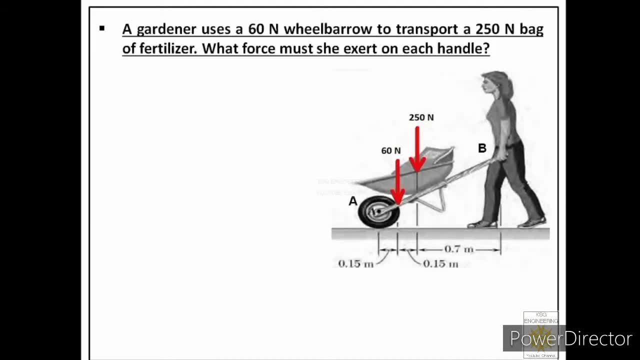 So I hope the solution of this numerical is clear to you. Let us start the next numerical. Let us read the statement first. A gardener uses a 60 Newton wheel barrow to transport a 250 newton bag of fertilizer. What force must she exert on each handle? So let us understand the diagram given to. 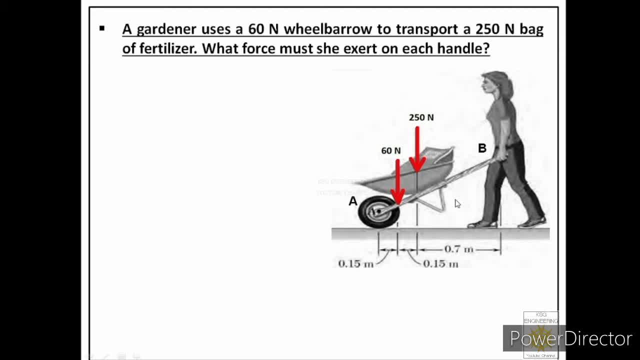 us. A gardener is transporting 川 a bag of dry Hieron 50 Newton through a wheelbarrow which is of 60 Newton, and both the forces are also labeled in the diagram and their distances from point A are also given to us. Point A is the centre of the wheel and point B are the handles. from where 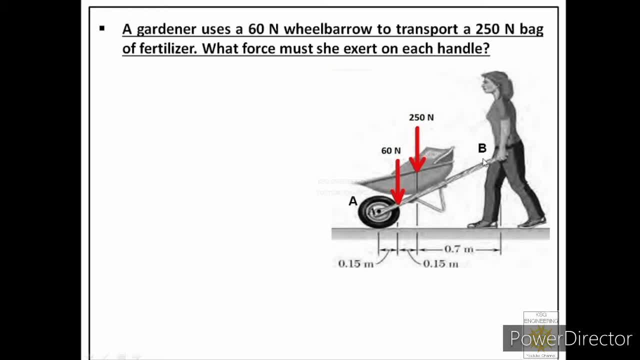 the gardener is lifting this particular wheelbarrow. Now what we are asked? we are asked to find what force must she exert on each wheelbarrow handle. remember, in this picture only one handle is visible to us, but there are two handles. so whatever reaction we will consider at handle B, that reaction will 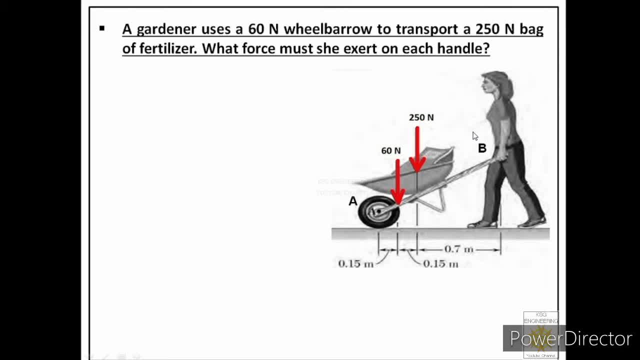 be for both the handles, fine, but reaction at A will be only one reaction because only one wheel is given for the wheelbarrow. now let us see how to solve this problem. so we know that in order to solve this problem, we have to sketch the free body. so how to sketch the free body? we will draw whatever given in the 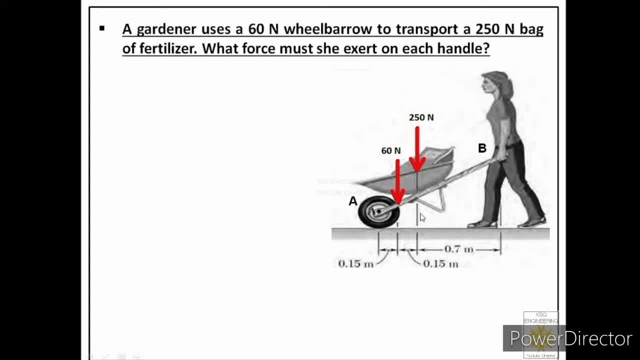 quotient. that means we will draw wheelbarrow, we will label all the important points, we will label all the external forces given and will label all the dimensions given. there is no need to draw the gardener because this is not a drawing class. fine, so there is no need of drawing of. 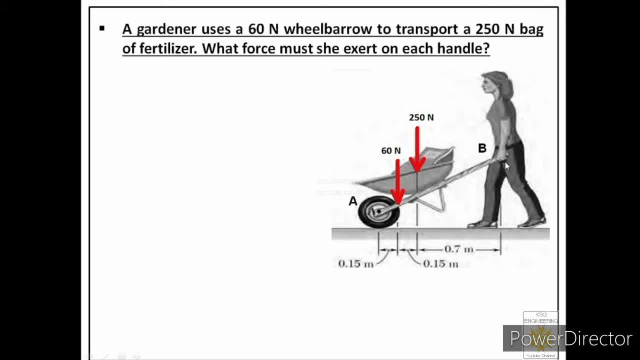 the gardener. you will only draw the body and we will represent the handles as point B. after that we will label the reactions. now let us understand carefully what will be the reactions in the free body and how to label those reactions. so for that we have to identify a. 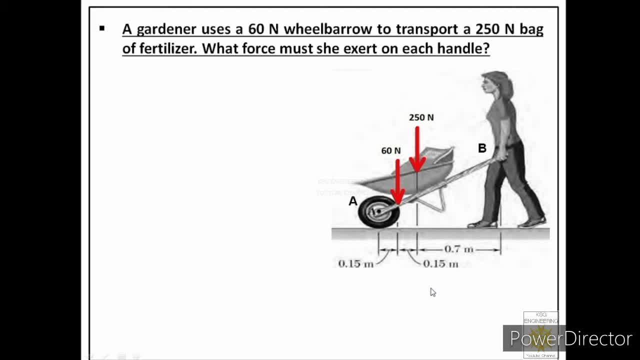 fixed form given to the existing direction of variation from the beginning. if we want a gave, a fixed form 같은 the fieldiggly situation. so the human action of measurements and Loudon's structure when situation is FIRST situation, unconscious deviation. there are two functions in a free body, like relationship and호. 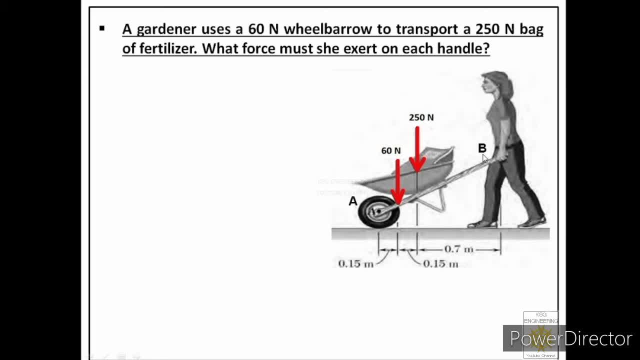 we will call it the best example, regardless of the tuttiys: safety. and the word of the orange, 순간knecher, means not united fit when situation consists like reactions will act at end B, but in the free body we have to show only one. but. 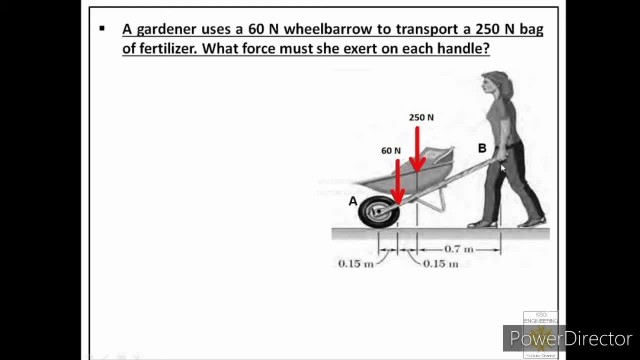 that one reaction, whatever magnitude, we will calculate. that is for both the handles. fine. so at B we have to show reactions in our direction. why? because Gardner is providing support at handle B to the wheelbarrow by lifting it in our direction. so let us show those reactions now. so at wheel we have shown one. 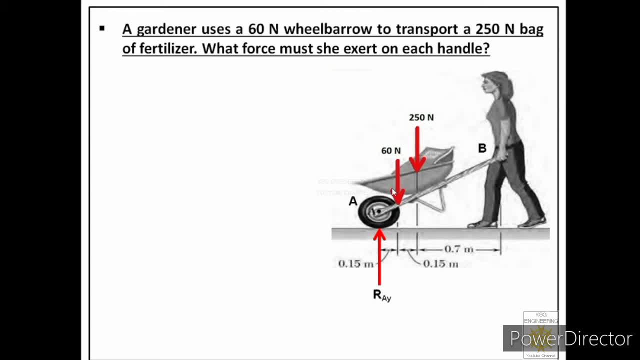 reaction that is normal to the surface because it is a ruler support. so we have labeled it as a reaction at A in Y direction. then we have labeled reaction at both the handles of the wheelbarrow as reaction at B in Y direction. now, first of all we have to say 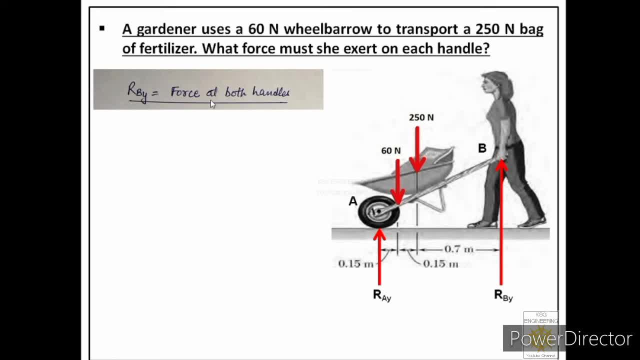 say, say, say, say that I am considering RBY as force at, or the reaction at, both handles. fine, this will keep in our mind, because in question he is asking us: what force must she exert on each handle? so when we will get the value of RBY? we have to divide. 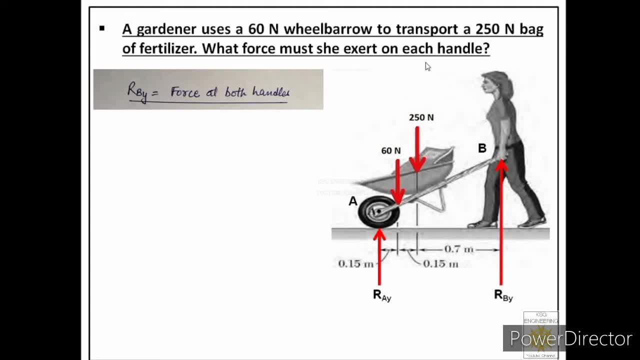 that value by two, to answer the question, because he is asking on each handle and this is for both handles. okay, so in this case again, we can say that this body is in equilibrium, it is not moving in X direction, it is not moving in Y direction and it is not rotating as 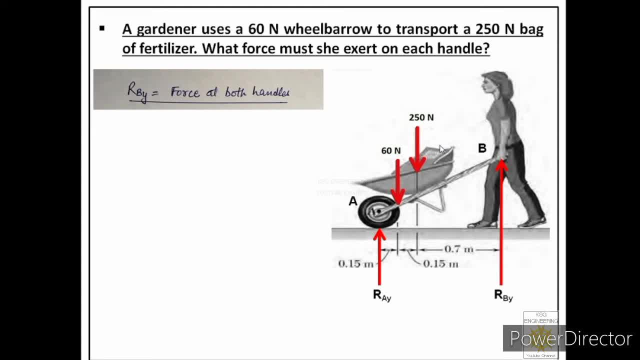 well. so three equations are applicable. those are: summation FX is equal to zero, summation FY equal to zero and moment at any point, because of all the forces, must be equal to zero. so let us start with the first equation: summation FY equal to zero. so how many forces are acting in Y direction? there are four forces. two are: 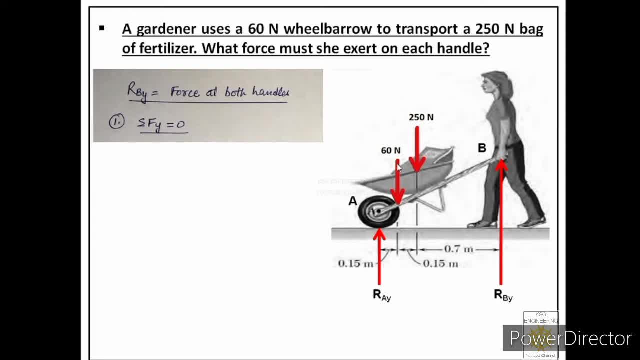 acting in downward direction and two are acting in upward direction, so these two will be taken as negative and these two will be taken as positive. so let us see this through calculations. so see over here: RAY minus 60 minus 250 plus 50, so RBY equal to zero. so in this equation we have two unknowns, so we cannot solve so. 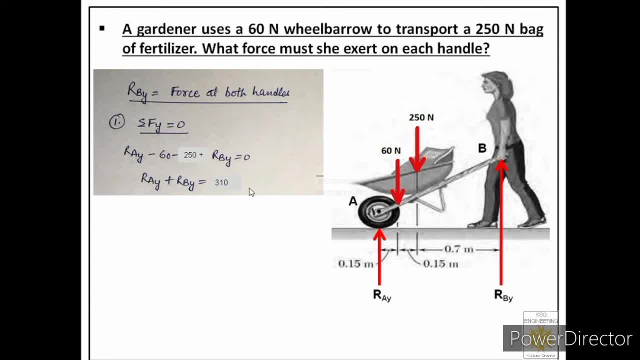 we'll name this equation as equation number one. next we will use another equation. that is moment. because of all the forces about any particular point must be equal to zero. see, we are not using summation. FX is equal to zero because in this free body there are no forces acting in X direction. so we are. 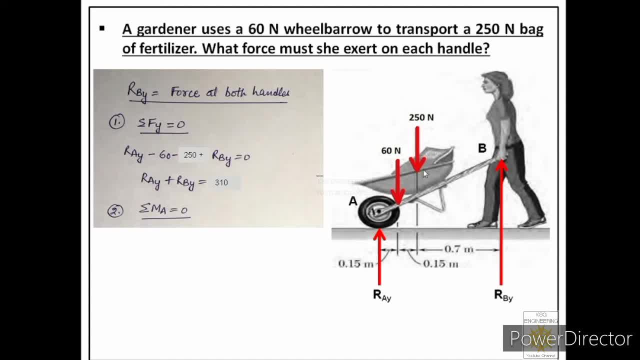 not using summation, FX is equal to zero. okay, now we have four forces and all the forces are acting at different points, so we can consider moment at any particular point. so let us consider moment about point A. so when you will consider moment about point A, then moment because of this force will be zero. 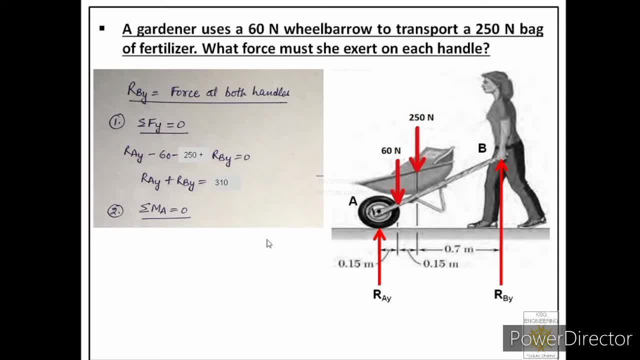 because it is directly acting at that point. so let us find the moments because of these three forces. let us first talk about this particular force and then we will consider moment because of this particular force. so this is the line of action of the force and from movement center this will be the perpendicular. 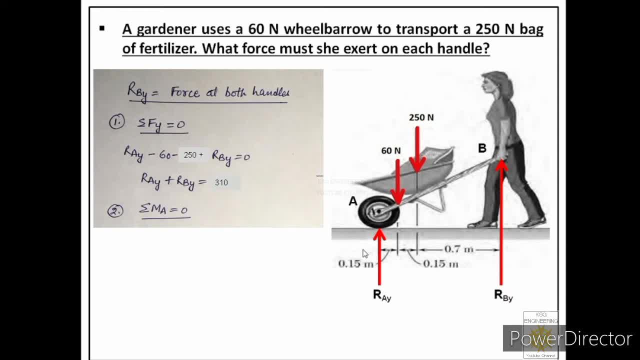 distance. so this is the moment arm. so this is labeled over here as 0.15 and the nature of this moment will be clockwise. so moment, because of this, will be minus 60 into 0.15. similarly, for this particular force, we will draw its line of action and from moment center will drop a. 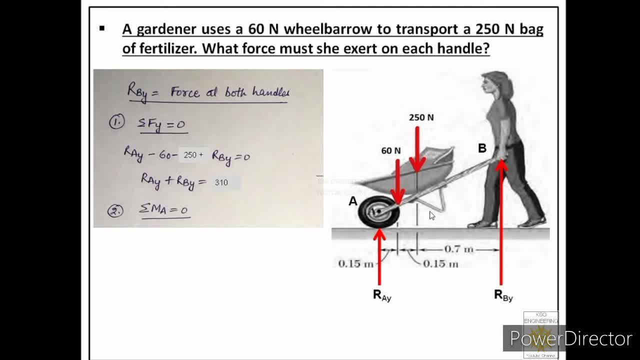 perpendicular. so that moment arm is labeled here as 0.15 plus 0.15. that is point, three meters. so it will also generate a clockwise moment. so we have to take that negative. so moment, because of this force will be minus 250 into 0.3. then we are left with this force. now this is the line of action of the force. 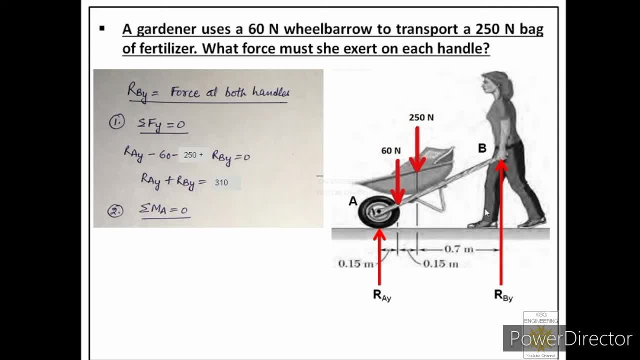 and from moment center. when you will draw perpendicular onto that line of action, that will become moment arm. so that moment arm is the sum of these three distances, that is, 0.7, 0.15, 0.15. so that will be equal to one meter, and the nature of this particular force is: 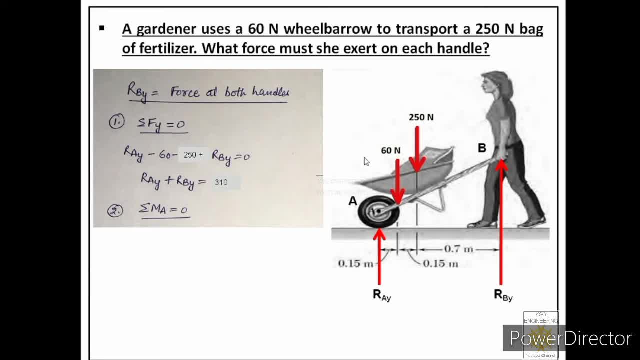 anti-clockwise. fine, so it will generate positive moment. so moment, because of this, will be positive rby into one meter. so let us see the calculations you can see over here: minus 60 into 0.15, minus 250 into 0.3, plus rby into 1 is equal to 0. so in this equation we have only one variable or one. 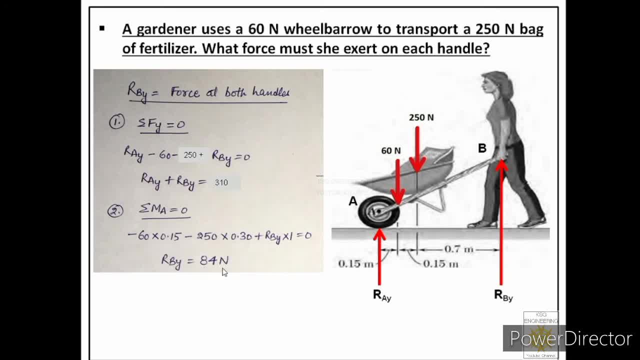 unknown and we can find that unknown. so it is equal to 84 newtons, a very important point to understand. 84 newton is the value of the reaction for both the handles, but we have to answer at each handle. so we will divide this by 2. fine, so we will get the answer as 42 newton as the force acting on each handle. so i hope this. 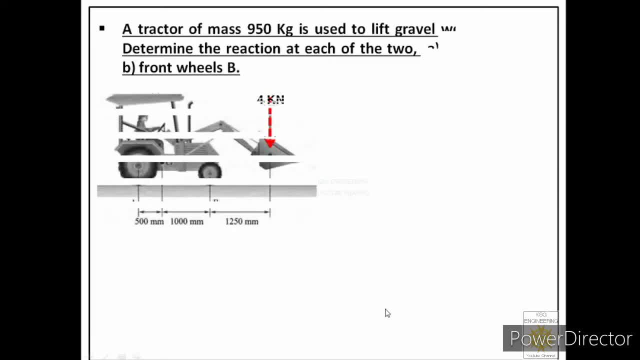 numerical is clear to you. let us solve one more numerical. a tractor of mass 950 kilogram is used to lift gas gravel weighing 4 kilo. newtons determine the reaction at each of the two: a part, rear wheels at a, b part, front wheels at b. so in this figure we are given one tractor and tractor has a mass of 950. 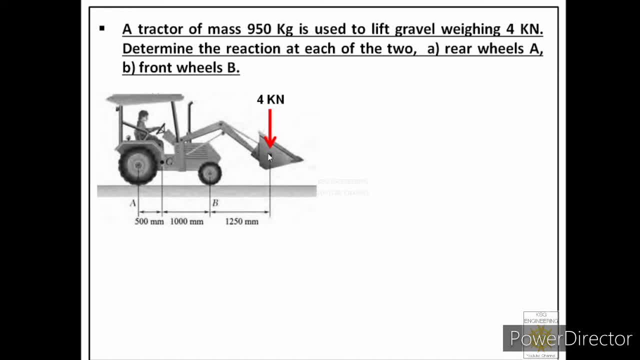 kilogram and it is lifting gravel weighing four kilo newtons. it is also labeled in the diagram. now, in this diagram, two wheels are visible to us, and these are rear wheels and these are front wheels. but we know that in a tractor there are four wheels. so at point a, we have to consider two wheels. at point b, we have to consider two wheels. now we are asked to. 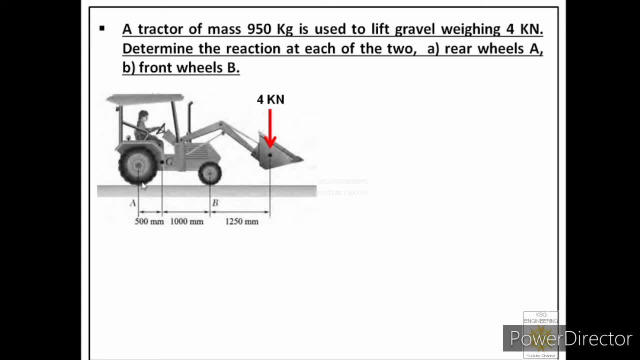 find reactions at rear wheels in A part and reactions at front wheels in B part, and we have to give the answer for each wheel. fine, now let us solve the problem. so, in order to solve the problem, we have to draw the free body. so we will construct the free body means we will draw a block diagram for this tractor. 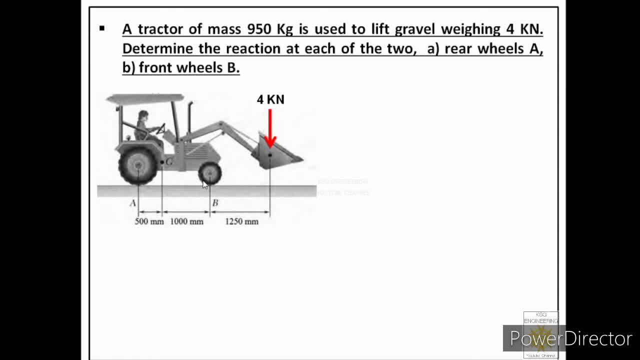 will show two circles below that block diagram and will label all the active and reactive forces on that free body. so let me show you here only so. we have two roller supports and we know that roller support provides only one type of reaction that is normal to the surface. so let us first label reactive forces at 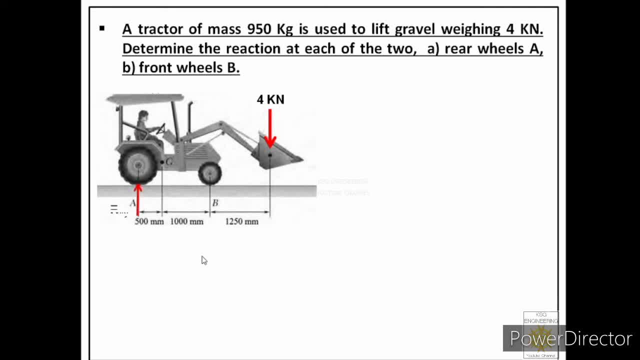 support A and at support B, so these two will be in vertical direction. so let us label it as reaction at A in Y direction, reaction at B in Y direction, and initially we don't know their direction, so we have assumed that these two are acting in upward. 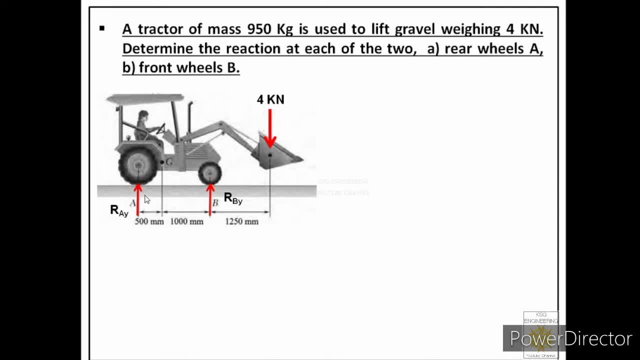 direction. so after labeling the reactions, we will label other external forces, and other external forces are already labeled in the diagram. so we will label the external forces, and other external forces are already labeled in the diagram. apart from that, we should label the weight of the tractor and it G, the 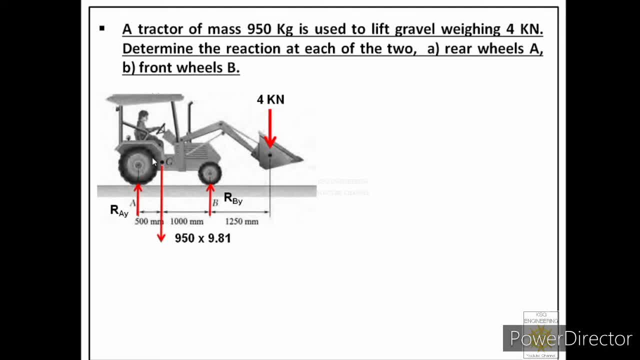 center of gravity is shown, so we will label weight at that point only in downward direction. mass of the tractor is given to us as 9.50, so we will multiply that by 9.81 to show the weight. now we are done with the free. 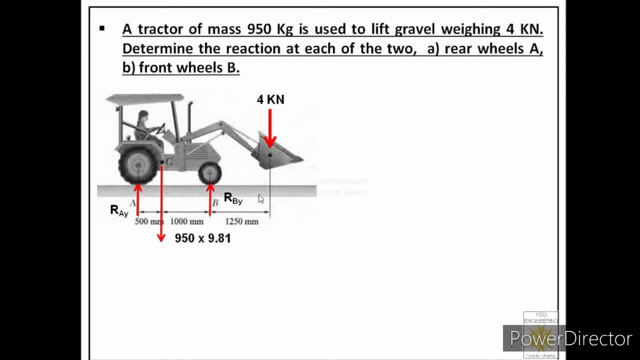 body and we know that the tractor is an equilibrium. it means all the three equations are applicable. summation: FX is equal to zero, take fewer than сб, quality is less, number than eat less and be less than whiter than and minus 3000 is less compared to km. Tracking temperature: Jacob Clarke t. and we know that the tractor is in equilibrium. it means all the three equations are. 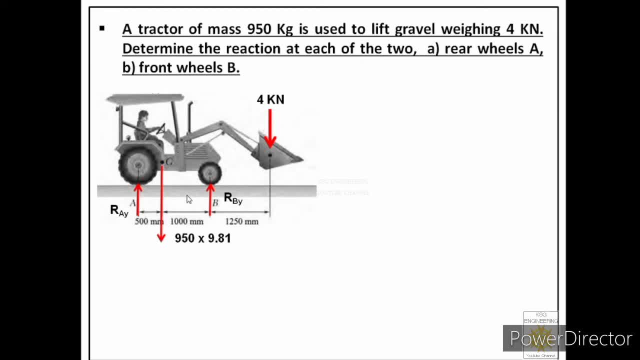 applicable, summation fx is equal to 0, summation fy equal to 0 and moment, because of all forces at any particular point, is 0. let us solve the problem. so before solving, we have to declare that we have taken RAY RBY reactions at. 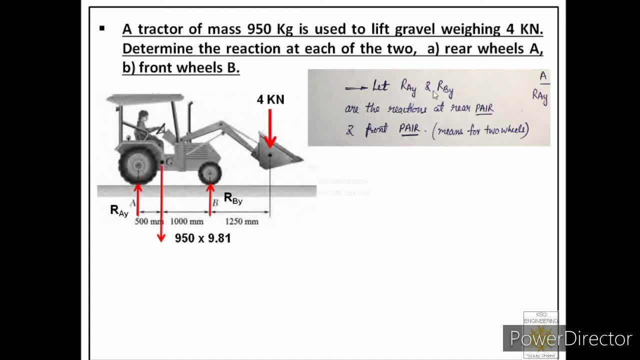 rear and front wheels and these reactions are for both the wheels means RAY is the reaction for both rear wheels and RBY is the reaction for both front wheels. now we will apply the first equation, that is summation. fx is equal to 0, but in this free body there is no horizontal force, so this equation is of: 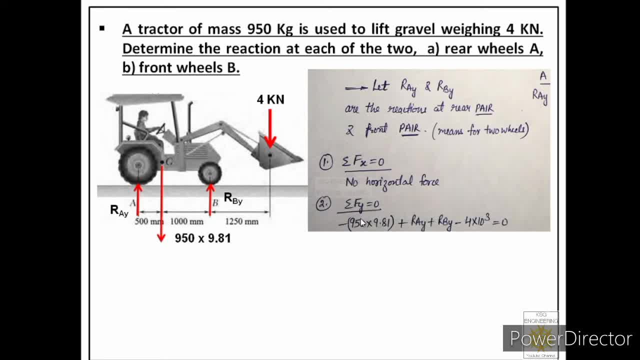 no use for us. now. let us apply the second equation, that is, sum of all the vertical forces must be equal to 0. we have four vertical forces and we have two vertical forces, and we have two vertical forces and we have two across our direction. these will be taken as positive and two are acting in. 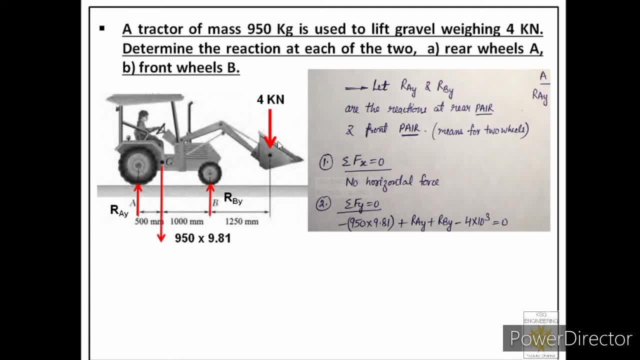 downward direction. so this will be negative. you can see over here we have taken minus 950 into 9.81, plus RAY, plus RBY, minus 4 into 10 to the power 3. why we have taken this? because it was given in kilo newtons but weight is in. 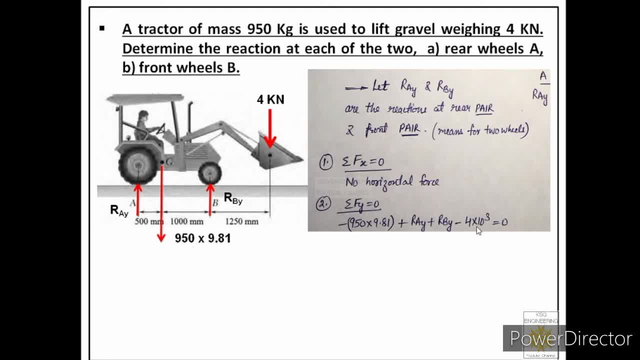 Newtons, so we have converted this into newtons as well. so in this situation we equation. we have two unknowns, so we cannot solve this equation, so we'll call that equation as equation one. now we'll apply the third equation, which is take moment, because of all forces at any particular point. so let us take moment. 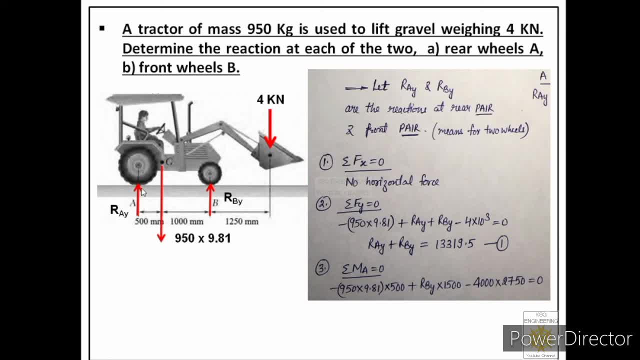 about a, as this reaction is directly acting at moment center, so perpendicular distance is zero, so there is no role of this reaction for the moment. when we consider at point A, now we are left with only three forces. so let us discuss one by one their moments. let us start with the weight now. this is the line of 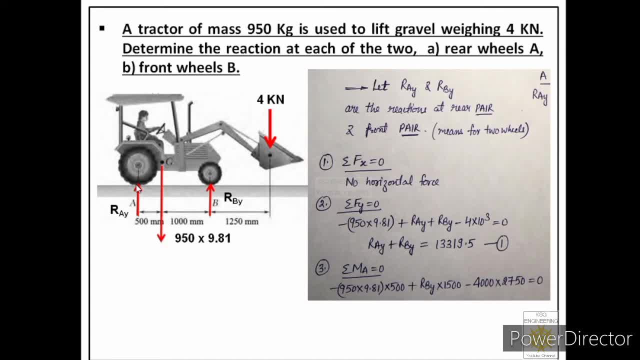 action of the weight and this is the moment center. so drop a perpendicular onto that line of action. so this is the moment arm. so this moment arm is given over here as 500 and the nature of moment generated by this force is a clockwise moment. so that will be negative. 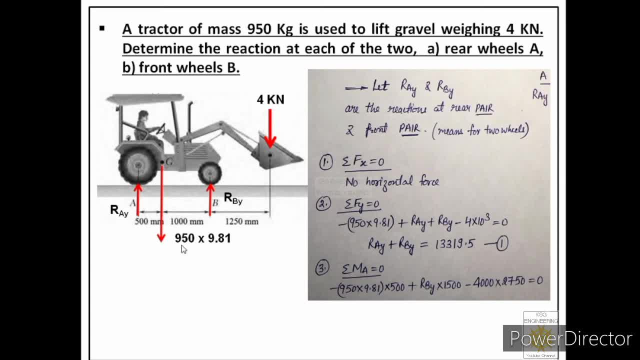 so its final moment will be minus 950 into 9.81, into 500. look over here: minus 950 into 9.81, into 500. and let us talk about the moment generated by this reaction, about a. now, this is the line of action of this reaction and this is the 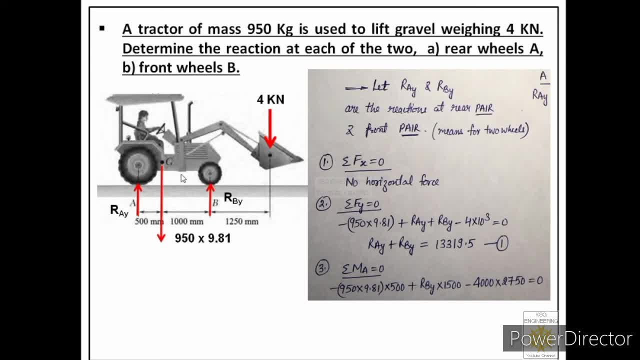 movement center drop a perpendicular onto line of action. so this is the moment arm. so this moment arm is the sum of five plus 1000.. So 1500 mm is the moment arm. Now let us see the nature of the moment generated by this. 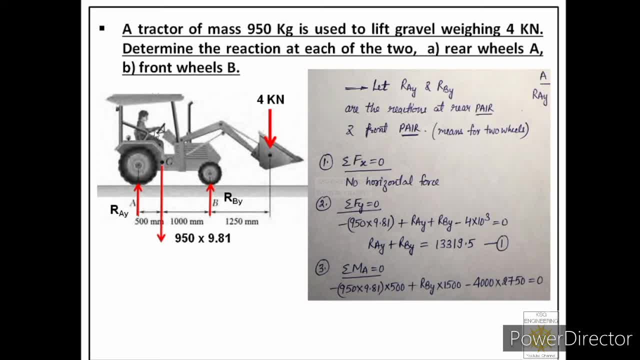 reaction. This reaction will generate anti-clockwise moment. So that will be a positive moment. So moment because of this will be plus RBY into 1500.. Look over here: plus RBY into 1500.. Now we are left with last force. This is the line of action of that force and this is the moment center. So from 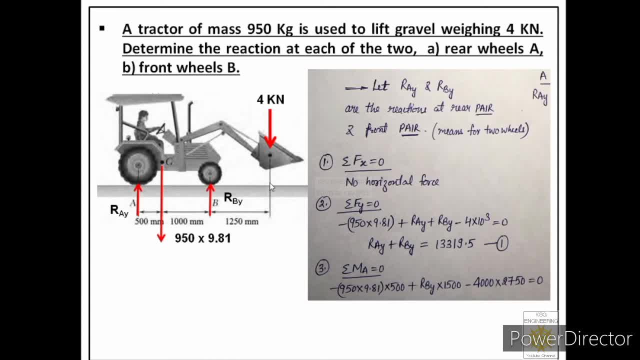 moment center draw a perpendicular onto that line of action. So this is the moment arm. So this is equal to sum of 1250, 1000 and 500, which is equal to 2750 mm. And the nature of this moment is: 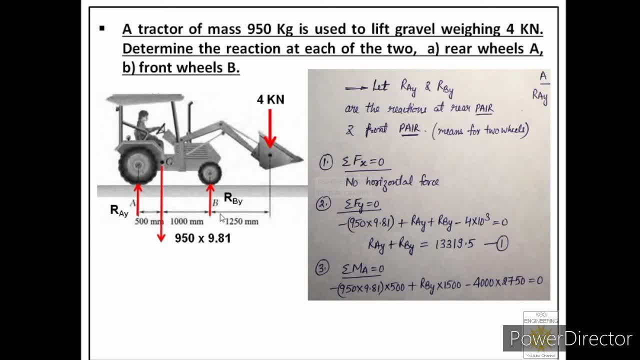 clockwise and it will be taken as negative. So moment because of this will be minus 4000, because we are converting this into Newton, into 2750.. Look over here: minus 4000 into 2750, equal to 0.. Now in this equation we have only one unknown. So we can solve that unknown. So when we 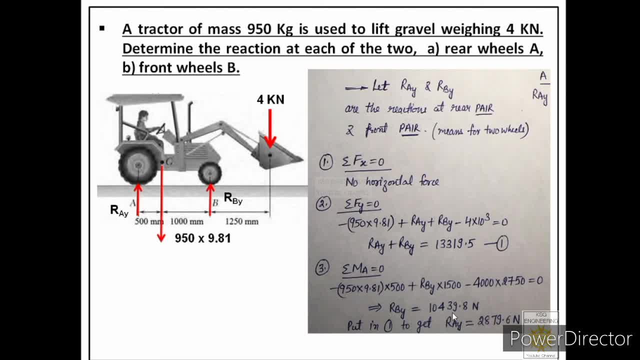 solve this equation, you will get RBY as 10439.8 Newtons And this is a positive value. That means the direction which we considered at the start of the numerical is correct. Now we will say: RBY is equal to 2750.. So we are converting this into Newton, into 2750.. So we are converting this.